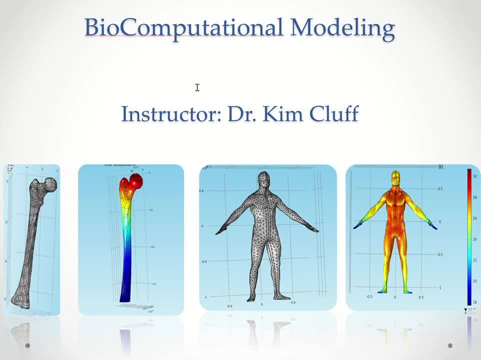 Okay, good afternoon. Let's go ahead and get started. So welcome back to biocomputational modeling. Today I'm going to provide a brief overview of what is biocomputational modeling. Let's go ahead and start with a quick review of what is biomedical engineering. 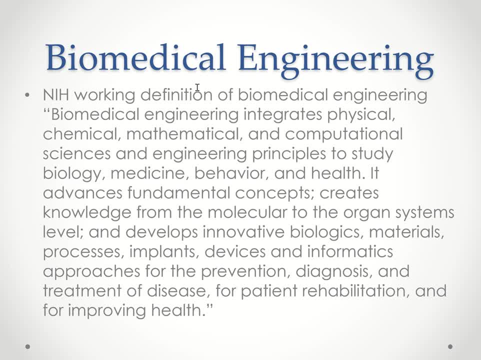 Well, if you look at NIH, the working definition of biomedical engineering is someone that integrates physical, chemical, mathematical and computational sciences and engineering principles to study biology, medicine, behavior and health, And it's someone who advances fundamental concepts, creates knowledge ranging all the way from the 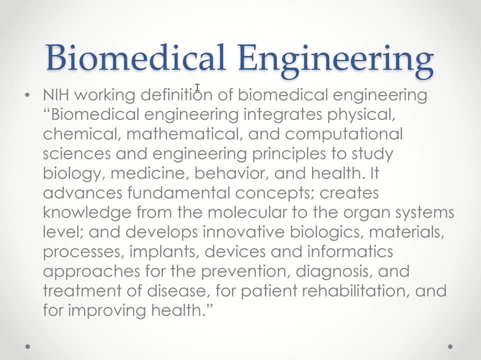 molecular to the biological, And it's someone who advances fundamental concepts, creates knowledge ranging all the way from the molecular to the biological, And it's someone who advances the molecular system all the way to the organ systems and develops innovative biologics. 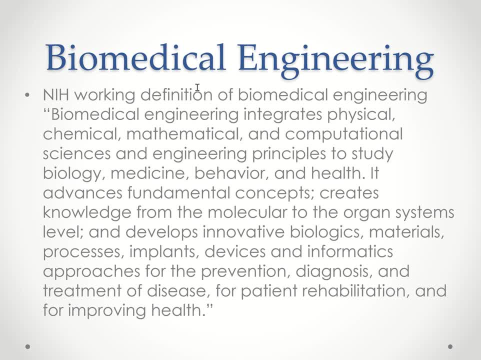 materials processes, implants- that would be biomaterials, devices would be medical devices like a pacemaker, and informatic approaches for the prevention, diagnosis and treatment of disease, for patient rehabilitation and improving health. So a biomedical engineer is very multidisciplinary engineering And again the computational sciences. 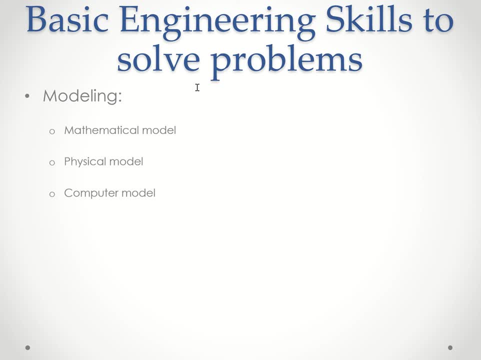 play a big role in it. So when we're talking about modeling, what kind of modeling are we talking about? There are several different ways you can model. In fact, there are three different ways you can model. There are three different ways you can model. There are three different ways you. 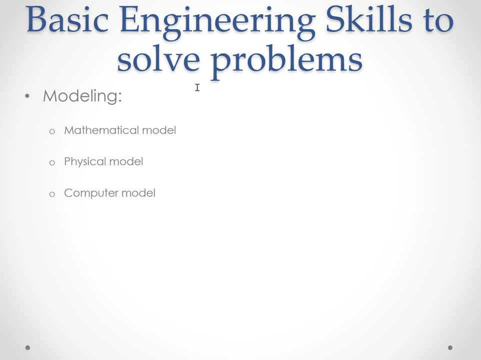 lack. Shall you tell them just in the knocked off Spanish, this kind of switch f? let's go back to thatyal working on a texted. Here's your tip, That is, you can do a model One, you can make a mathematical model. Okay, that includes. 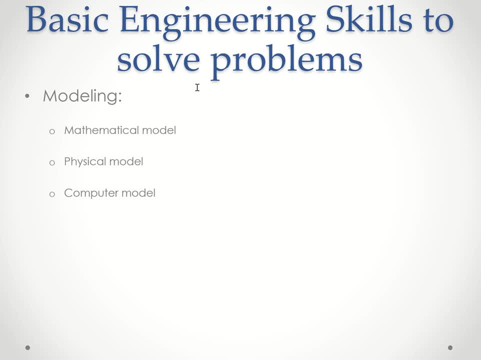 Mathematical equations. They're trying to approximate The world around us. The world around us, or the system that you're trying The world around us, or the system that you're trying to trying to model and make, Get results based off of calculations, Was. 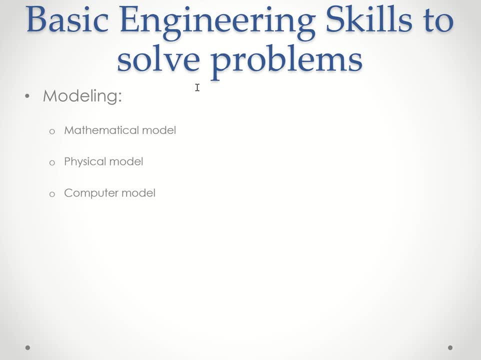 maybe a small-scale prototype, and try to physically model the system and get results from it that way. the third way is to use a computer or a computational model. okay, now, in a computational model, that's what will be. that's the type of modeling we'll be doing in this class, where we use a computer to solve all the 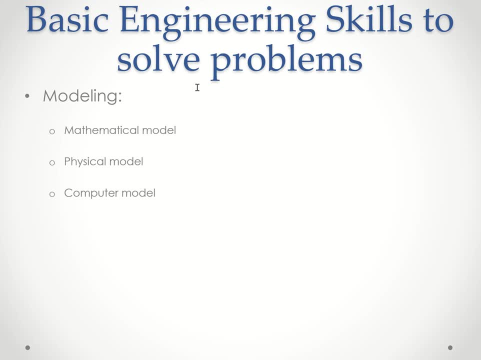 equations for us, the differential equations for us and where. but we have to set it up, okay. and something important to note about models: okay, is that all models are wrong, but some are useful. okay, that's an important saying when it comes to computational modeling, and the model is only as good as the 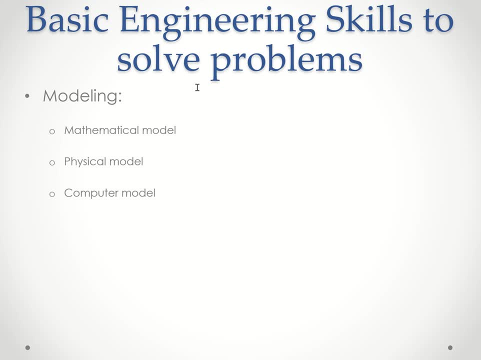 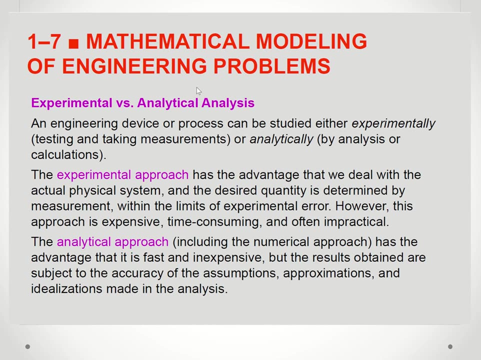 assumptions you make and like that. okay, so let's talk a second about mathematical modeling versus physical modeling or experimental model modeling. okay, so again, an engineer- I can, can study systems either experimentally by taking tests, by making tests and taking measurements, or an engineer can study the system mathematically with a. 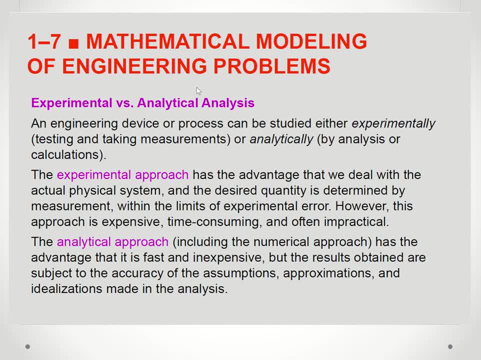 mathematical model, by analytically or analyzing the situation with equations and calculations. so in both have their pros and cons. okay, the physical model or the experimental approach has an advantage that you deal with the actual physics system- okay. and the desired quantity is determined by the measurements of that. 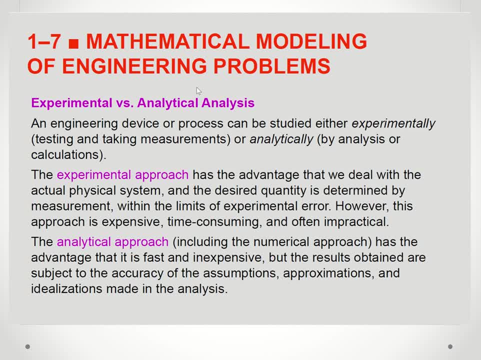 and it could be, you know, scaled down prototype, a smaller version, and so that's the benefits of an actual physical model is that you can make measurements from it, okay. one of the downsides of this type of modeling is physical modeling is that it's it can be expensive, okay, and it can be. 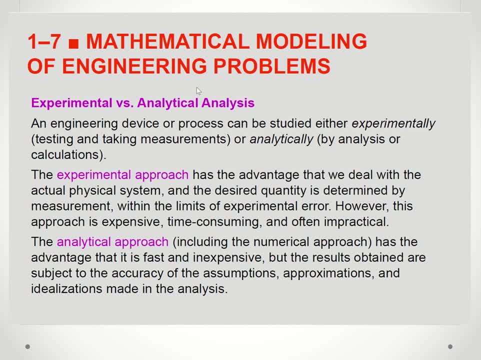 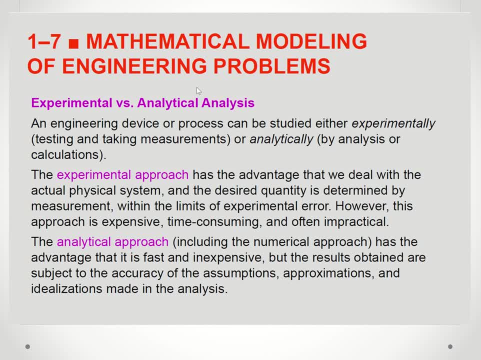 all, even impractical to do. if you want to model something inside the human body, you might not be able to physically do it, so the other approach is this analytical approach or this mathematical modeling approach. okay, so this approach includes, you know, numerical equations and calculations, and one of the advantages 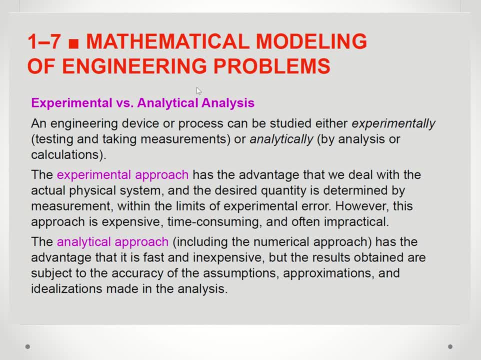 of it is: it's fast and inexpensive, especially if you can just do it on, you know, pen and paper. one of the downsides of it is oftentimes the results are subject to the accuracy of your assumptions or your approximations and how well your equations model the real world. 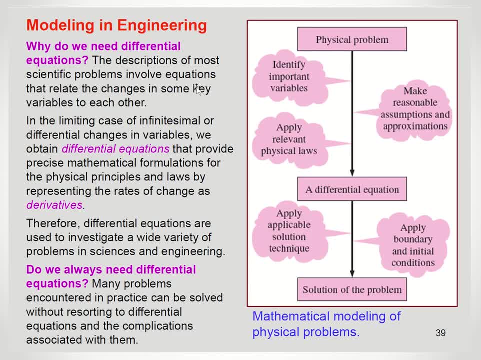 okay, so the basic workflow when it comes to modeling is: you start with some sort of physical problem that you want to model And you take a look at the problem and identify what are the important variables that govern or change in the physical problem And then, based on that, 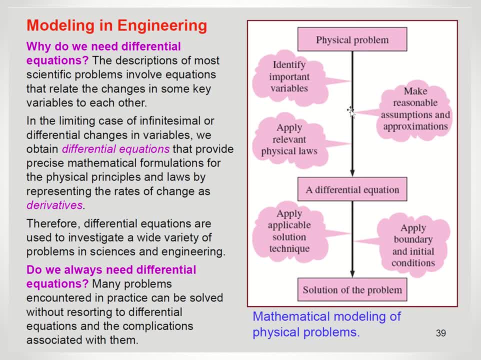 you make assumptions and approximations And then you apply the relevant governing equations based on the physical laws. That typically leads to a differential equation And then you can apply an applicable solution technique to the differential equation and apply different boundary conditions or initial conditions and solve the problem. 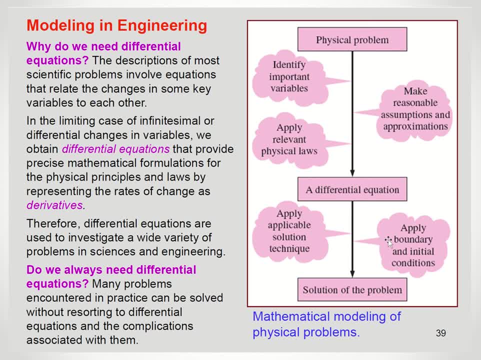 And you have. You end up with a solution to the problem. Okay, So in this process, differential equations is often very important. The description of most scientific problems involves equations that relate the change of some key variable to another key variable. Okay, 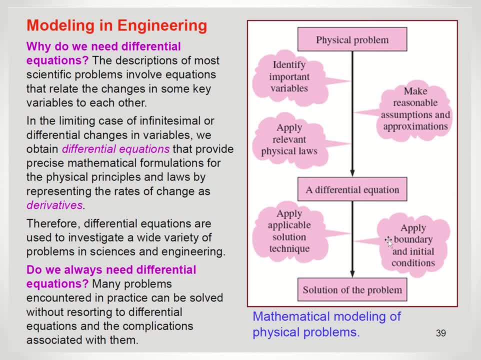 So this is what differential equations does for us, And a lot of the governing equations do involve differential equations. However, some problems, or many problems that we encounter, can often be solved without resorting to differential equations as well, But again, the accuracy will depend on the assumptions. 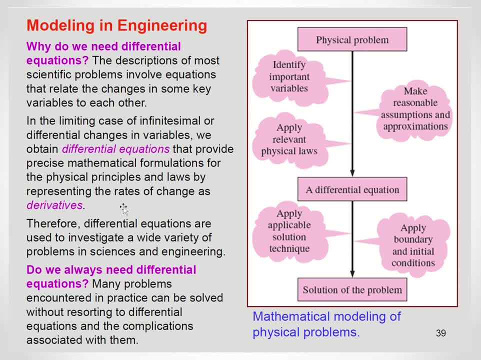 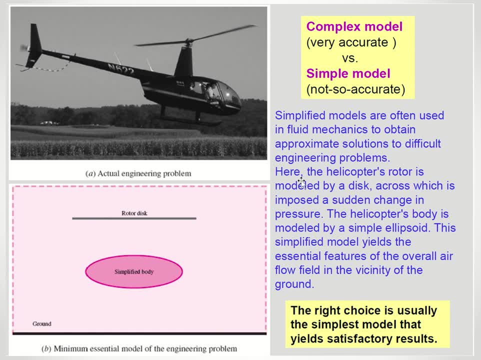 and approximations that you make. Okay, Let me give you an example here of a model. So let's say we wanted to model a helicopter flying in the air, So that's going to include, Actually, that could be a very complex model. 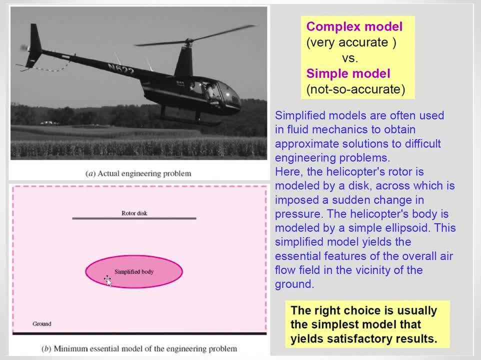 Or it could be simplified into something as simple as an elliptical body and some rotor nose. Okay, Okay, So when it comes to modeling, you can either have a very complex and very accurate model, or you can have a simple and not so accurate model. 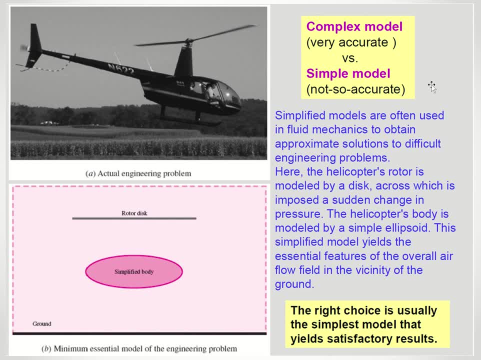 Both of those have pros and cons, So the simplified models often used to obtain approximate solutions. So for a simple트 to very difficult engineering problems. In this example, this helicopter's rotor is modeled just as a disk. Okay, flow, and but it'll be, it'll be, it'll have some errors because it's simplified. 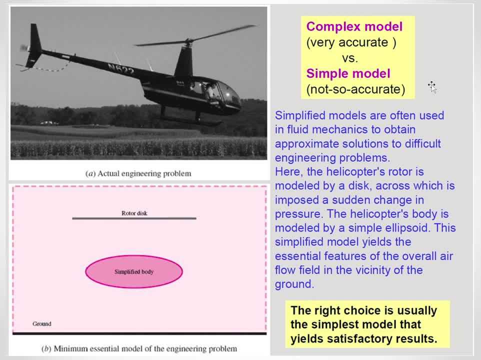 right. so the more complex you make your model, the more accurate will be, but oftentimes that it will come at a cost: a cost in terms of complications and and when it comes to computational modeling, it'll come at a cost of computational resources, and so, typically, the right choice is usually to select the 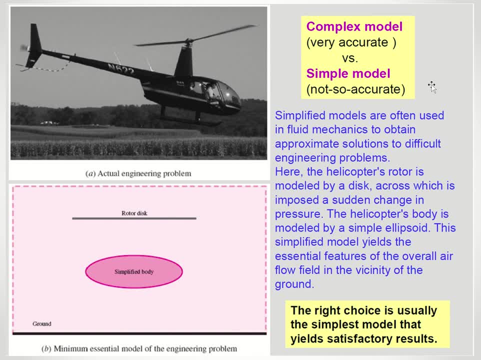 simplest model that yields satisfactory results. okay, so, and that's up to you, as an engineer, to decide what is the simplest model that will give satisfactory results. does it need to be so complex, or can it be simplified? do we need super high accuracy or do we need just ballpark numbers, or do we just? 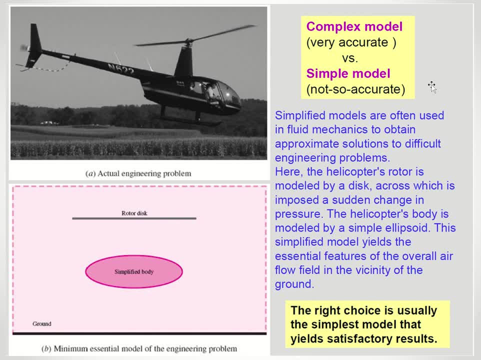 need to know that the helicopter is not going to fall out of the air and it'll stay up. so again, you can make a complex model, you can make a simple model. okay, both of those apply to whatever type of modeling you're doing. if you're doing a, 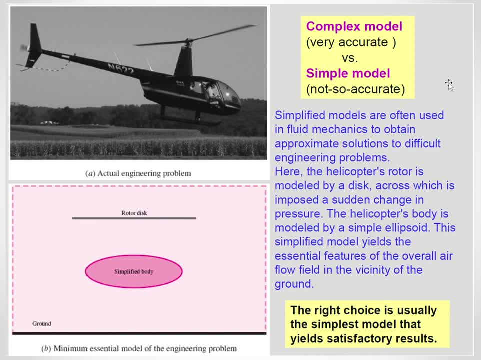 mathematical model. you can make it very complex with very complex different differential equations. if you're doing a physical model, you can make, you know, a physical prototype of a helicopter and make it fly, or or, or you can make a computational model and build it in in a 3d virtual environment in a computer and 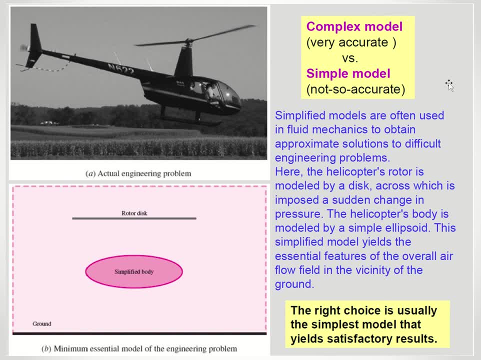 add many physics to it and make it complex, or you can make it simple. okay so, actually making it, making it the right choice, is a very complex model, and the way we can make it the right choice is usually to make a simple model that yields satisfactory results. okay so, and again, that's, that's actually a skill to. 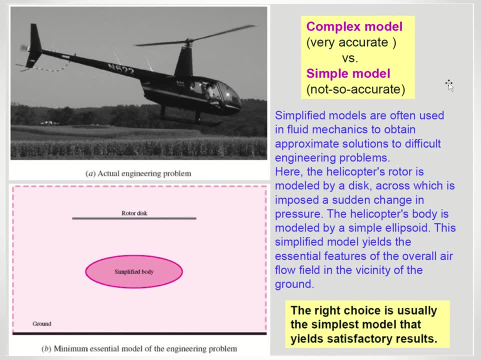 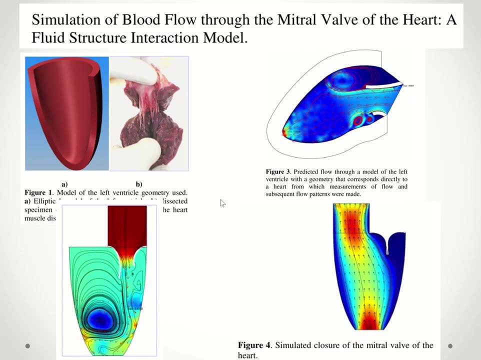 be able to judge and determine what is the right model based on the results we need. okay, so let me give you a couple of examples of other things that we can model. so here's an example of modeling a ventricle or blood flow through the mitral valve and in the 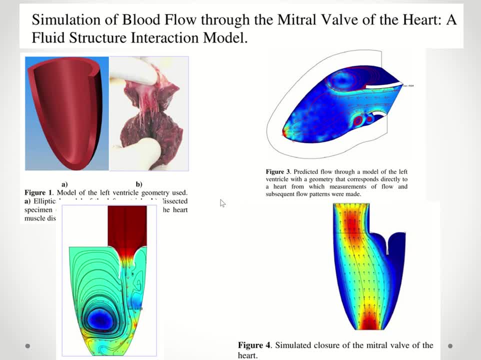 ventricle of the heart. okay, so again, this model could be very, very complex, or it could be simplified into something as simple as this elliptical geometry here, which simulates the ventricle inside the heart, and it could even be further simplified as a 2d model. 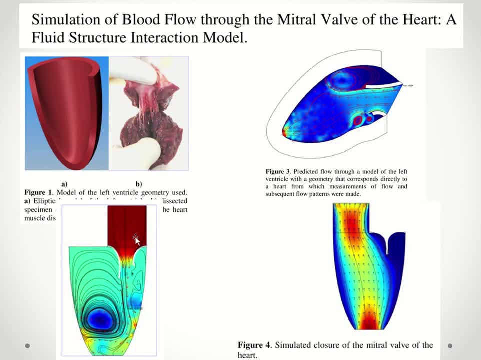 here, where this is the ventricle of the heart, this is the blood flowing through the ventricle and flowing through the mitral valve. here, as the mitral valve opens now, this, this approach, greatly simplifies the model greatly. so, again, it will be less accurate, but the question is: how accurate do you? 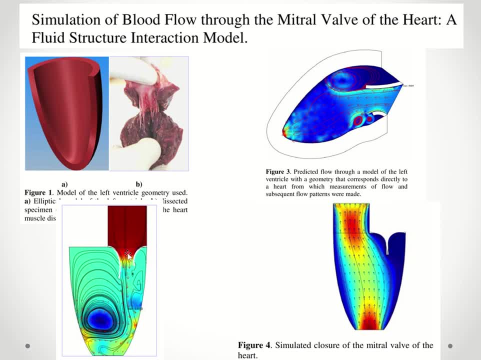 need to be. you need to be super accurate, or do you just need to be able to make judgment calls on certain parameters? okay, here's another example of simplifying ventricle of the heart. this would be the heart wall, the muscles of surrounding the ventricle. this would be the, the ventricle cavity and blood. 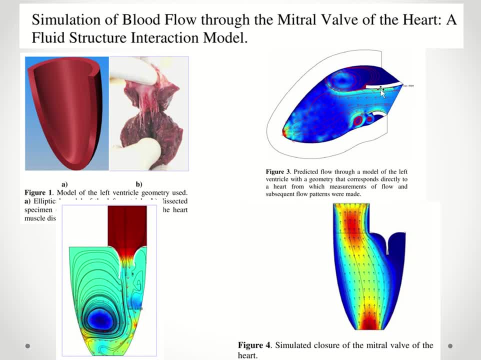 flowing in through the ventricle cavity and blood flowing out of the ventricle cavity is the blood that flows in through the when the valve is open and here would be blood flowing out of the valve. I believe this is the mitral valve, so this is the left ventricle of the heart and flowing. 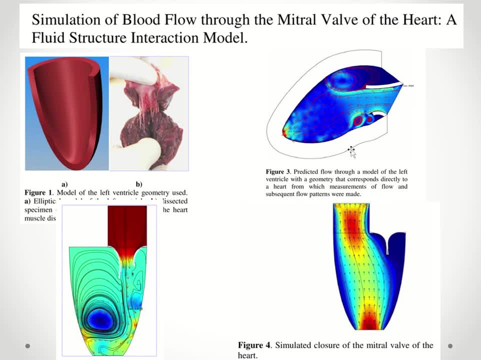 into the aortic artery, in the aortic arch, here, as blood flows. so, again, this is just a. this is an example of something you could model and how you can model it, and you can make it very complex, or you could think of how, ways to simplify the model and, again, like I said earlier, it's a skill to be able to. 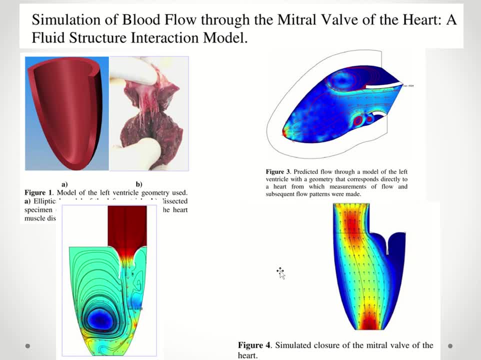 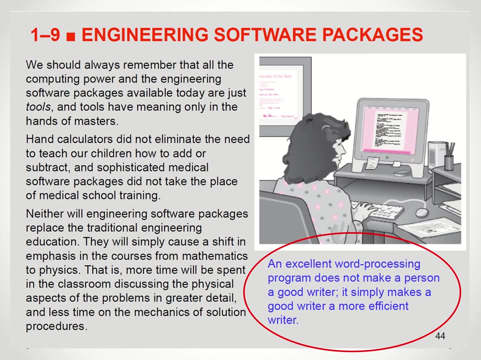 simplify the model and identify, okay, what are the important parts that need to be modeled and what are the less important parts of the geometry that can be left out, and how accurate do you need to be? okay, so again, like I said earlier, all models will be wrong, but some are useful. okay, just like mathematical equations may not. 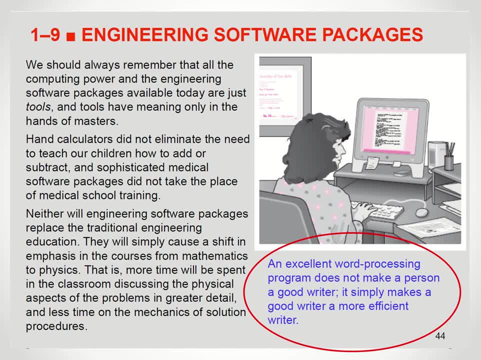 completely accurately model the world around us, but they're useful, right, so we use them okay, and when we need to be more accurate, we get into more complex differential equations- okay, and so what's important to remember- is that here's a good example- is that an excellent word processing program will not make a 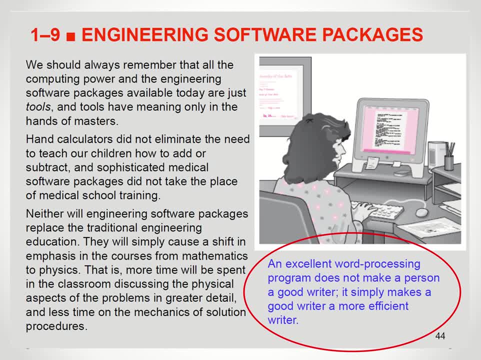 person a good writer: okay. it simply makes a good writer more efficient. writer. same thing with models: okay. or same thing with computers: a good computer and a good modeling software won't make a good model or make a good engineer. instead, it just makes a good engineer more efficient. 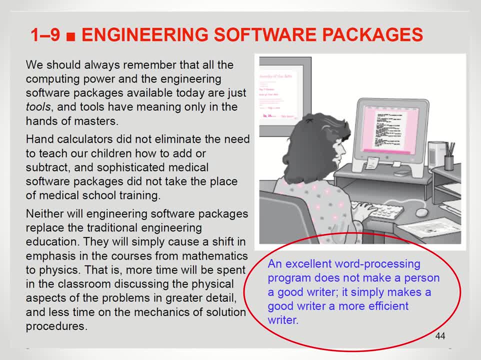 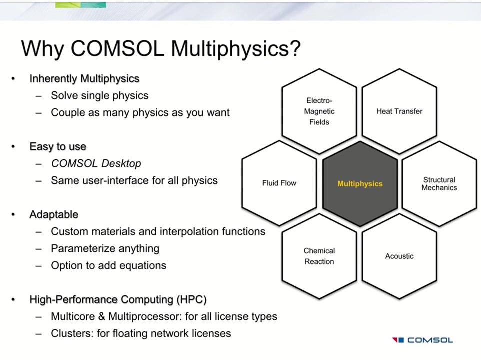 okay, so fundamental when concept when it comes to modeling, is that the modeling software is just a tool. okay, and the engineer has to have a good understanding of the physics and the governing equations and what they're trying to model in the software. okay, all right. so, uh, the type of modeling software that we're going to be using in 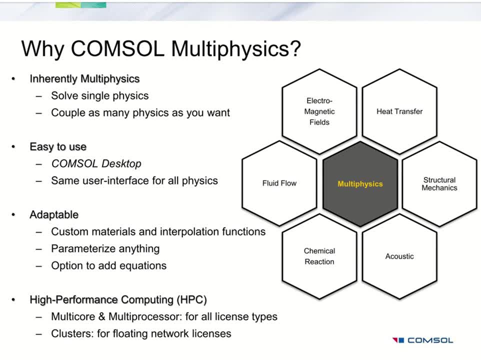 this class is, uh, comsol multiphysics. so why are we using the comsol multiphysics? well, it's a, as the name suggests, it's a multi-physics modeling software. it has the ability to model multiple different types of physics, including heat transfer, fluid flow, structural mechanics. 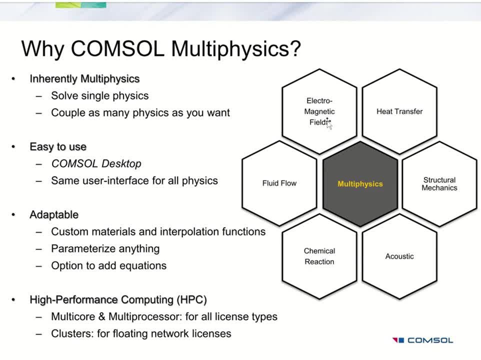 acoustics, even chemical reactions and electromagnetic fields. in this class we'll primarily just work with structural mechanics, fluid flow and heat transfer, but again com, the reason we're using comsol is because it's a multi-physics modeling software and it's also um fairly easy to use. it has a 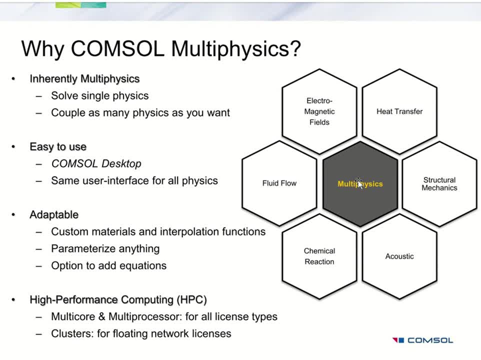 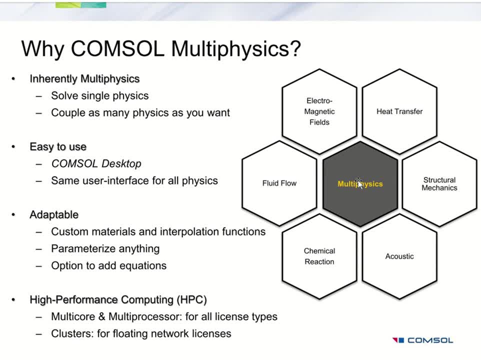 make a certain geometry, or make a certain geometry or that you want to model. it could be a simplified 2d geometry or or it could be a more complex 3d geometry, and it allows you to set up and apply the physics, the different boundary conditions and model it. 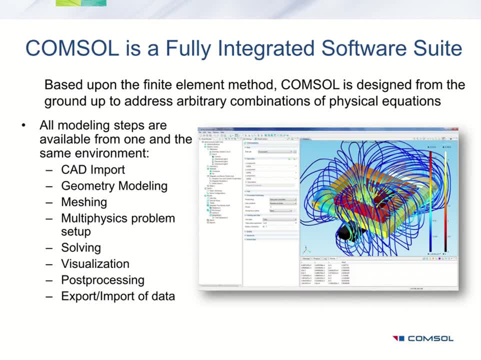 okay, so again, comsol. the general workflow when it comes to comsol, how it's how it works, is based on this finite element uh method. okay, so finite element analysis is where the geometry is broken into a whole bunch of tiny pieces in which the governing equations are applied. 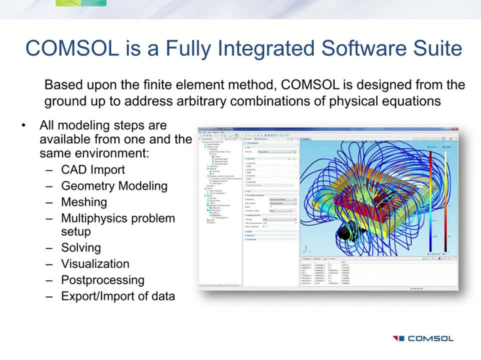 to each of these finite elements, and the basic workflow or the basic steps when it comes to modeling is: first, you bring in the geometry, that's the cat importation- okay, you bring in the geometry. you have to make a Accessorized Function, the Kirby's ư. 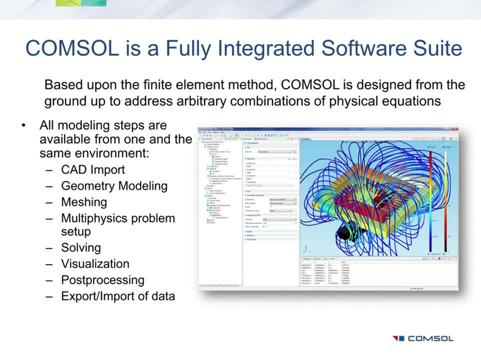 you have to make afs to just follow a given geometry and then you solve this cause. you get a. We'll be using SOLIDWORKS combined with COMSOL and we'll make some geometry in SOLIDWORKS and import it into COMSOL and I'll show you guys how to live, link those and work with them that way. 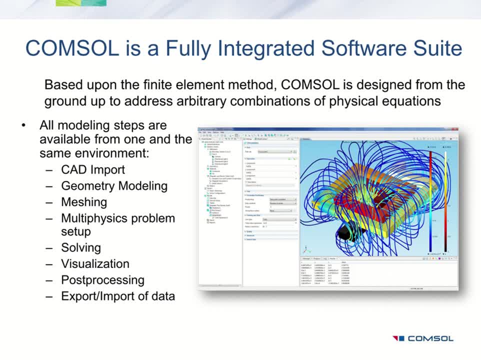 We'll also just work in COMSOL and I'll show you how to make geometry in COMSOL, and both 2D and 3D as well. The basic steps is to first bring in the CAD geometry or make the CAD geometry. Then we can mesh the geometry again, and COMSOL makes this very simple. 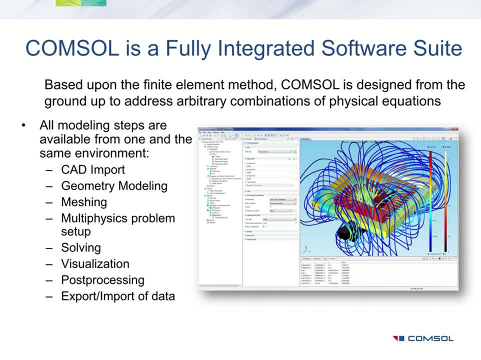 in that it's just another step in the process, Whereas, in reality, finite element analysis can get very complex very fast, And so COMSOL simplifies it greatly in that it's just a number of steps that you have to do and it will do all of the finite. 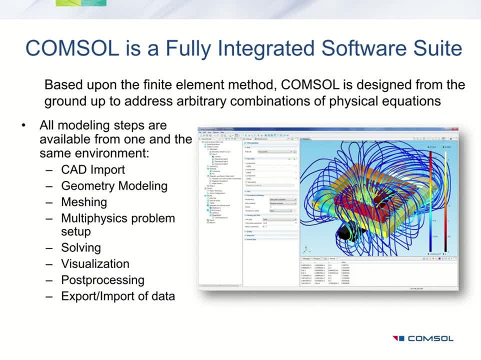 element analysis for you. okay, The next step would be to set up the physical problem. okay, That involves the physics, applying boundary conditions and initial conditions, and then solve it. And again, the model, because this is a computer like a calculator- will do the solving. 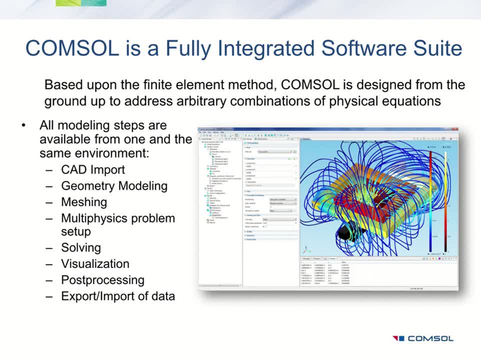 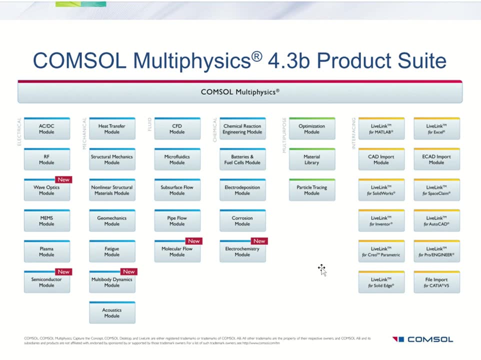 for you and then allow you to visualize the results and then do any post-processing and export the data. Again, because COMSOL multi-physics is a multi-physics modeling software, there's a whole bunch of different types of modules that you can use to model. Now we don't have all these modules, okay, So there's an RF module. 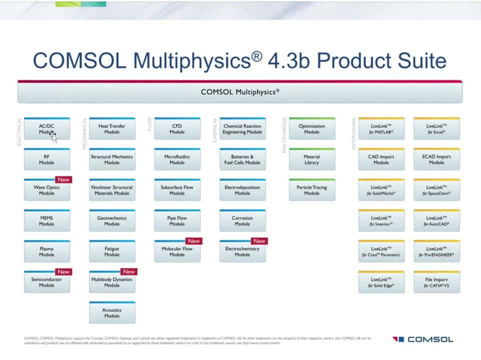 there's a wave optics module, an electrical AC-DC module. So we don't have all these modules, but we do have the heat transfer module. we do have the heat transfer module and we do have the heat transfer module, have the fluid dynamics module and we have the structural mechanics module. so 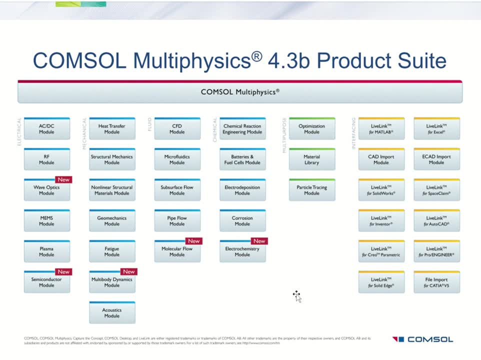 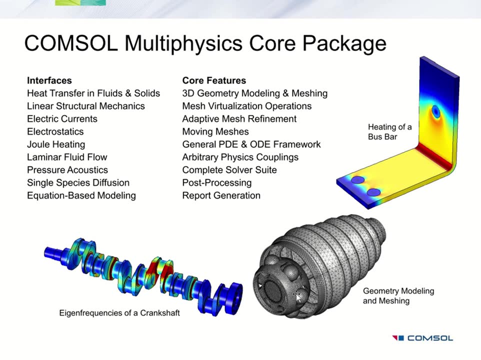 those will be the ones that we focus on mostly in this class. okay. so also that the console comes in a base package- okay, which allows you to do most of this modeling at more of a entry. entry level or elementary level basic modeling on all types of physics. to get it deeper into any kind of physics you need to 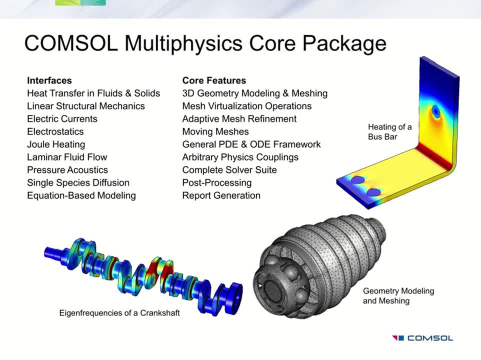 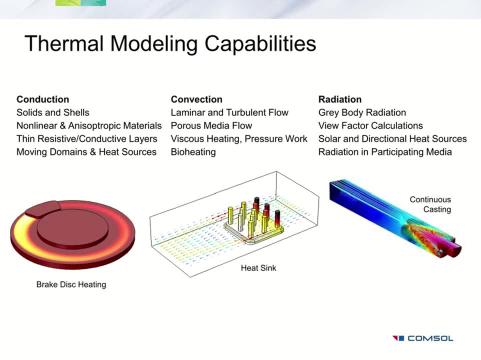 have a specific package that goes with it. so let me give you a couple of examples of the different type of modeling. so here's an example of some of the thermal modeling capabilities. you can see here that we have a lot of different models that we can use to model. 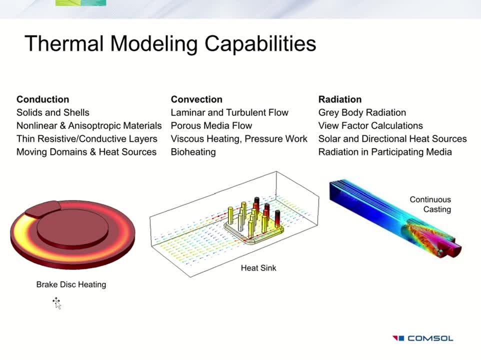 here's an example of say you wanted to model heat transfer on the brakes of a car- okay, so these are the disc, the disc heating on a car when the brakes are applied. or say you wanted to model heat transfer on a heatsink inside of a computer- okay, you could do. you could do this and set up fluid flowing over these. 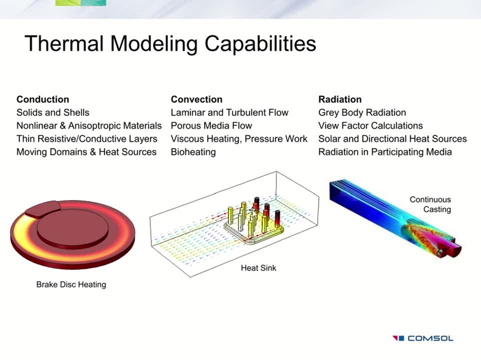 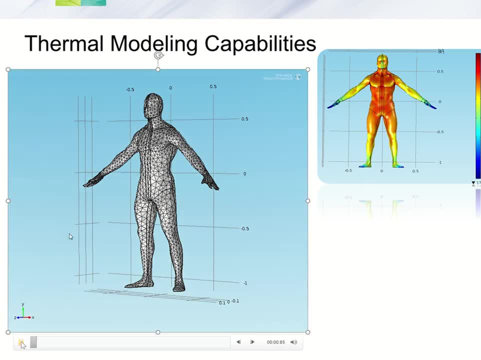 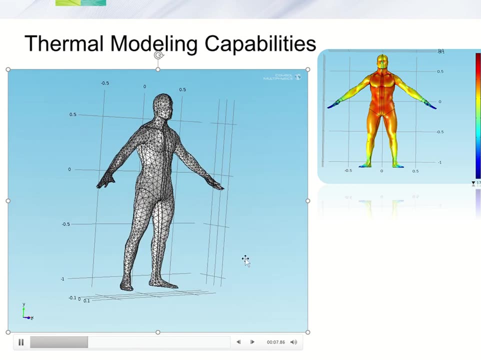 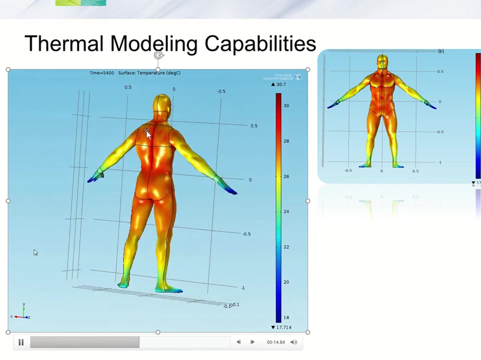 pins and the heat coming up through these pins and you can model that. here's an example of biocomputational modeling, trying to model heat transfer in the human body. this is actually an example of one of the homework assignments that we'll do in this class, where we apply heat transfer and model heat in the body. 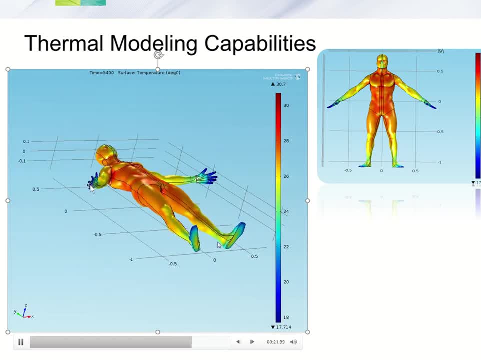 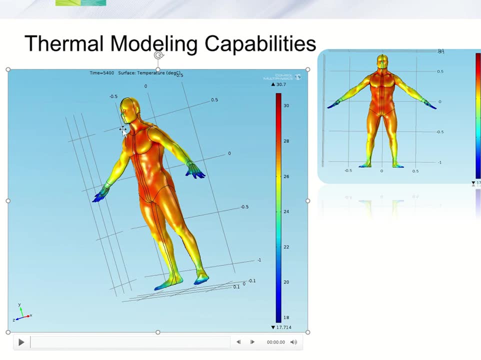 you can see here how we can model heat transfer in the human body. you can see here how we can model heat transfer in the body. you can see here how you can model heat transfer in the body. you can see here how the fingers are colder and the toes are colder, the Core is warmer. and again we can, we can apply this to different. 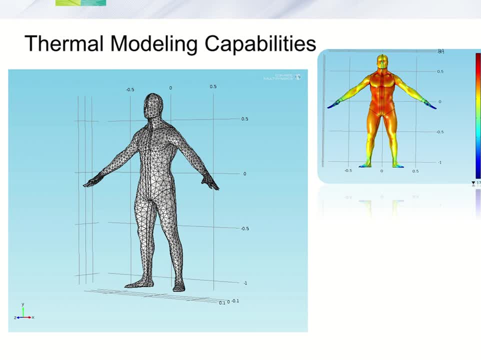 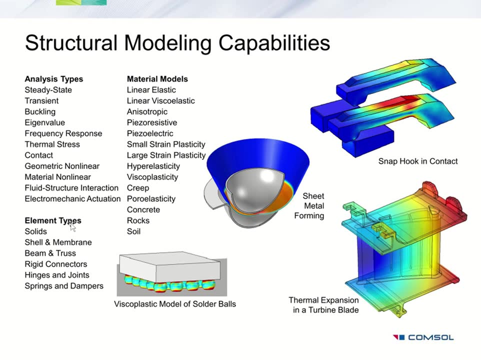 types of question is to solve different types of problems. another example of structural mechanics: modeling. okay, and you can model both you. you can model things like a steady-state structural mechanics, that's where the sum of the forces equals zero, or the model, the structure, is not moving. you can also even model transient state mechanics- okay, that's. 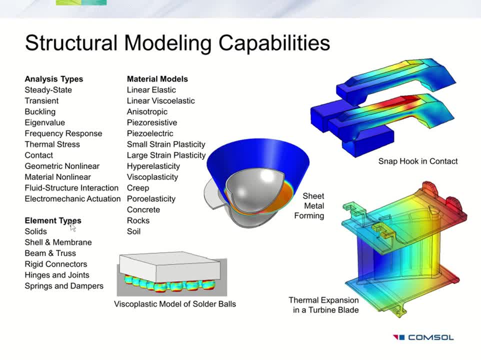 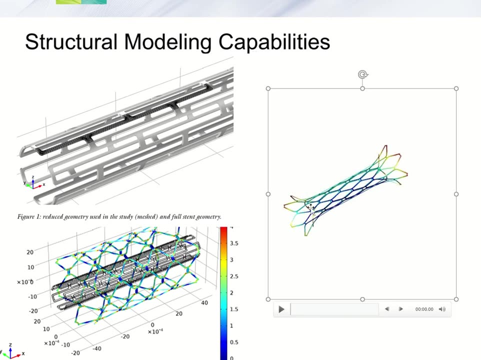 where something is moving. okay, it's the sum of the forces. in that case, it doesn't equal zero. okay, and let me show you some examples of some structural mechanics. this would be an example of modeling a stent that would go inside the artery. so stents are often used in patients that have aphosclerotic or 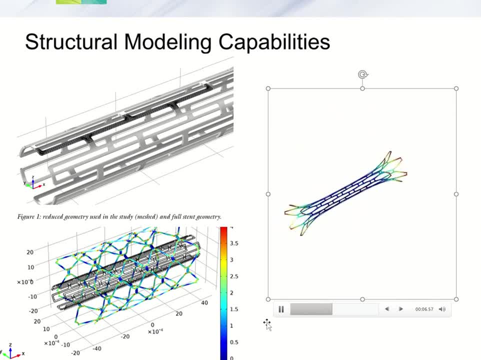 plaque buildup in their arteries, they'll often insert this stent and balloon in it, like it's shown here, and open up the artery. okay, and it'll hold the artery open. so this is an example of modeling some structural. this is some structural modeling capabilities in COPSL: modeling some structural mechanics and. 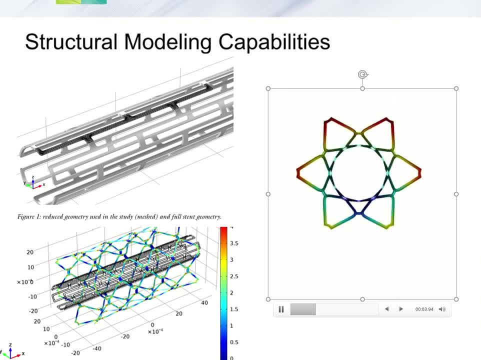 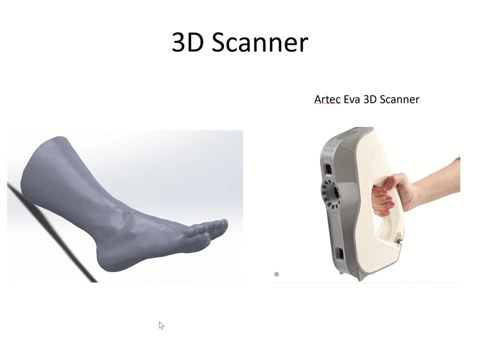 elastic properties of a stent that would go inside the artery of a patient with aphosclerosis. here's another example. you could use even 3D scan a patient specific geometry. For example, this is someone's foot in our lab that we scanned. 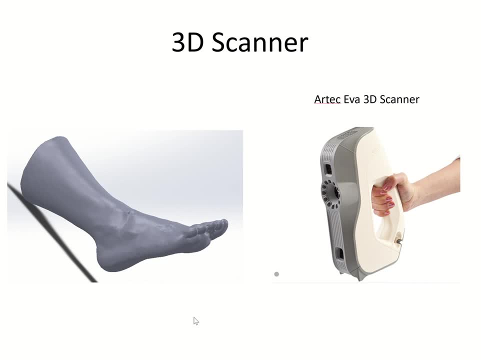 And you could bring in this geometry into COMSOL and you can start applying physics to it. And so say, you wanted to model a prosthetic or an orthotic, a brace that would go around this person's foot and how it would work. 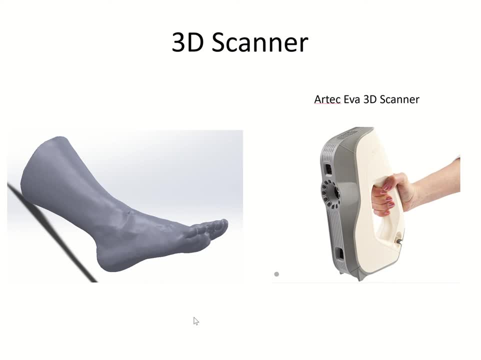 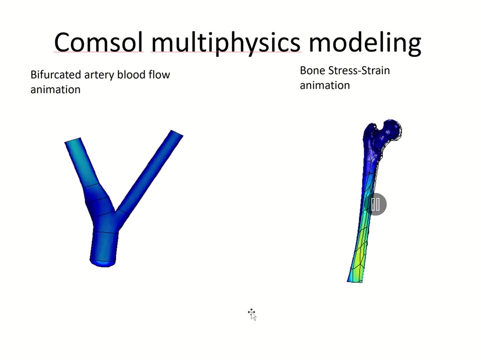 You could do that with COMSOL by first scanning the patient specific geometry and then bringing it in, And you could also even bring it in from like an MRI scan or a CT scan or different things like that. Here's another example of blood flowing through a bifurcated artery. 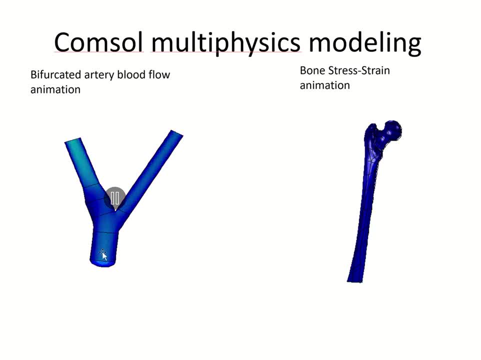 Okay, here's an example, And this would be an example of a non-steady state or transient state: fluid flow mechanics, because blood flowing through our body is not continuous, right? Instead, it's pulsatile Every time your heart beats blood. 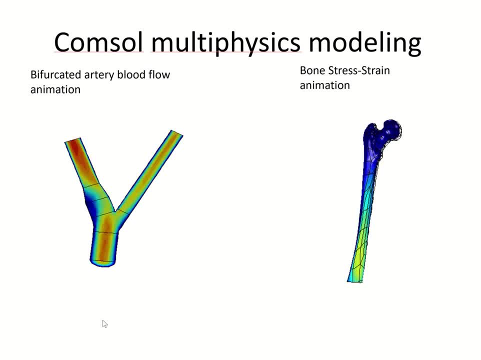 your heart pulses through the arteries and veins, And so this is an example of modeling fluid flow through an artery. Same thing if you wanted to model stress and strain on a bone or a human femur. Okay, actually, when you walk, the bones actually flex a little bit. 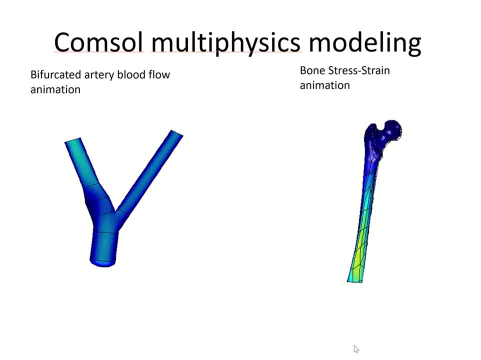 They bend a little bit under the load, okay, And so to do that, you need to do some work. So to model it, you could actually model this and measure the different stress and strain on the bone. Okay, here's another example of that: structural mechanics. 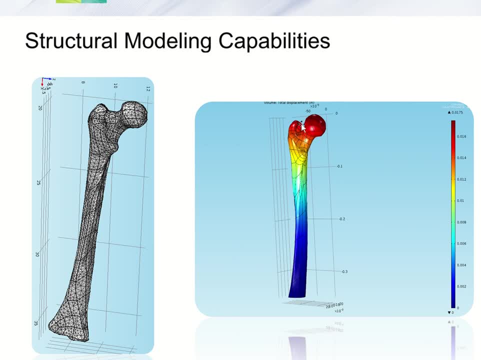 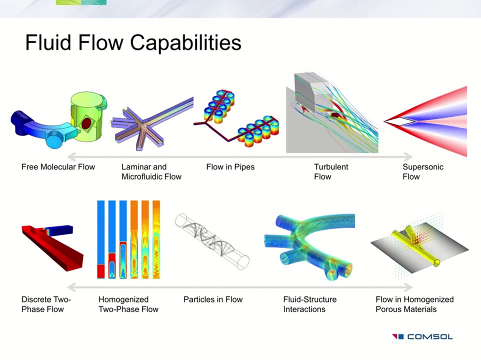 Say, you wanted to build an artificial hip that might go in here and see whether or not it'll hold up when a person walks. Okay, so those are just some examples. Here's some other examples of fluid flow capabilities. Again, you can model flow in pipes. 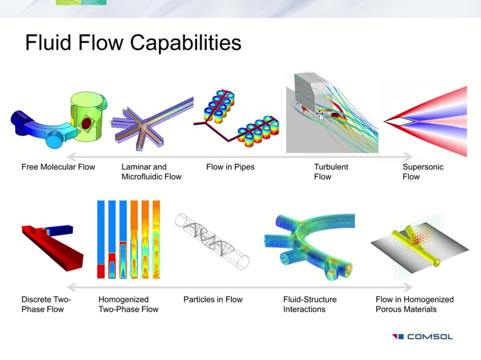 You can model flow around an object. You can model, do something, some kind of modeling called fluid structure interactions. Okay, this is an example of modeling the aortic arch that comes off of the human heart and breaks into the different arteries that feed your neck and your arms. 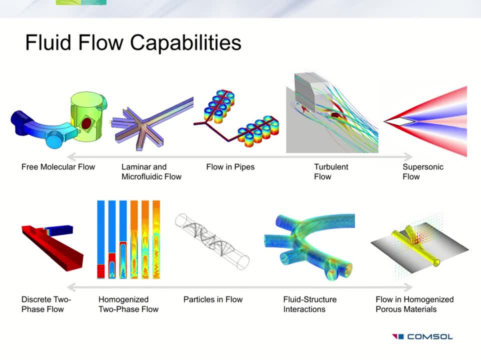 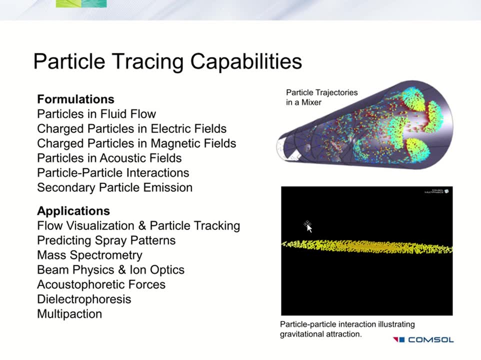 brachial arteries and carotid arteries. You could even do some particle tracing modeling okay, Where, if you have some chemicals mixing together, you could model how those particles and those chemicals would mix together And then you can visualize the fluid flow. 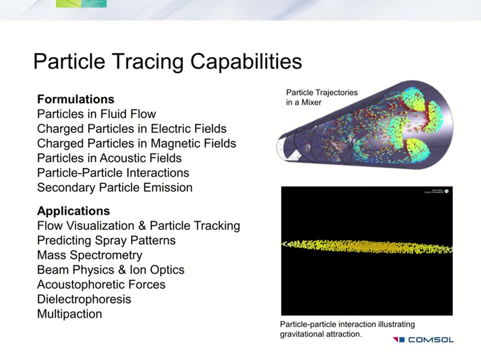 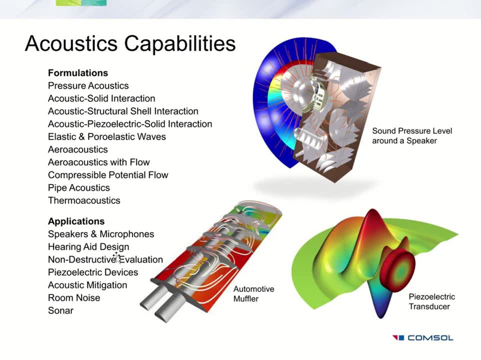 and do something called particle tracing as well. COMSOL also has the capability of modeling acoustics. okay, So acoustics are really nothing but pressure waves, mechanical vibrations in the air, So you can actually model this. So this is an example of modeling sound pressure levels. 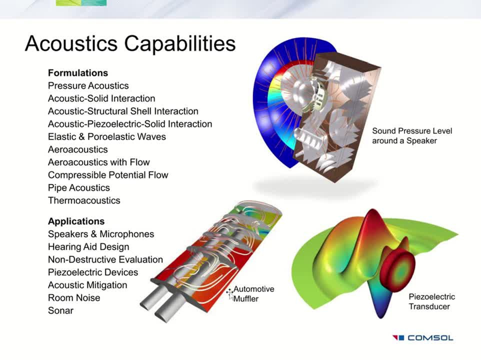 around a speaker- okay. Or you could model a car muffler- okay. So the muffler makes the car sound, it muffles the sound of the engine. right, And say: you wanted to make a better muffler. Well, you could do that in a model, in a computational model.